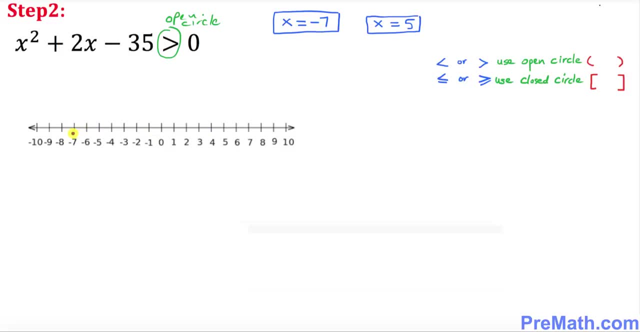 and see where our negative 7. so negative 7, and we know that's going to be open circle. I'm going to put down: negative 7 has an open circle and positive 5 has an open circle as well. that's the very first thing you must do. the next thing I want to make sure over here, whenever you have an greater than 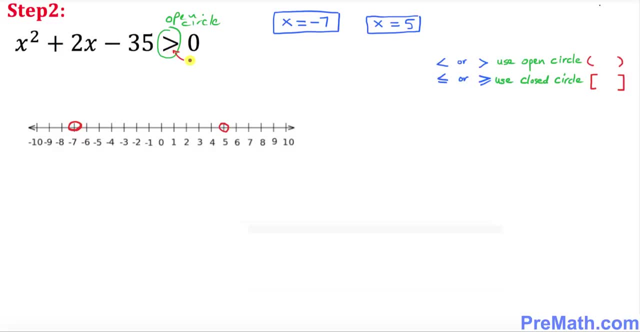 sign- always remember greater than means- is going to be opposite direction. so that means our graph is going to go the in the opposite direction. one is going to go this direction and the other one is going to go in this direction. so that means this side is going to be simply you. 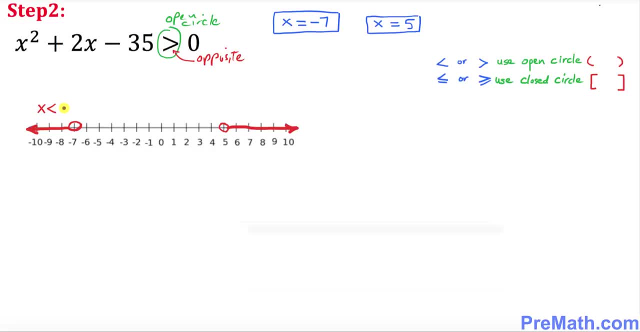 going to say x is less than negative 7. and here is going to be, obviously x is greater than positive 5, and our solution is going to be a. simply, you just put down these two inequalities. I'm going to put down x is less than negative 7, then you put r over here and then x is greater than 5. this is your solution. 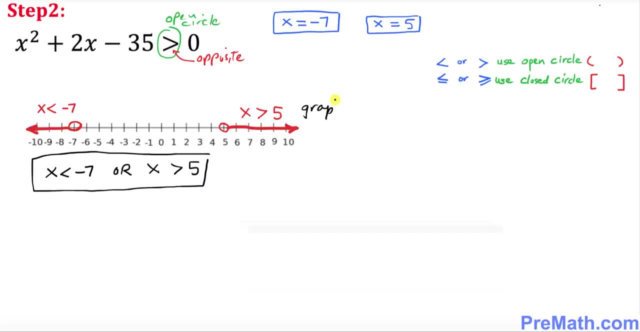 and, and this is our graph. Now, if you are wondering why these are going opposite directions, here is the justification I can give you briefly, And let me give you a justification over here. Here is our x-axis and this graph represents this quadratic function. okay, And now, as you can see, 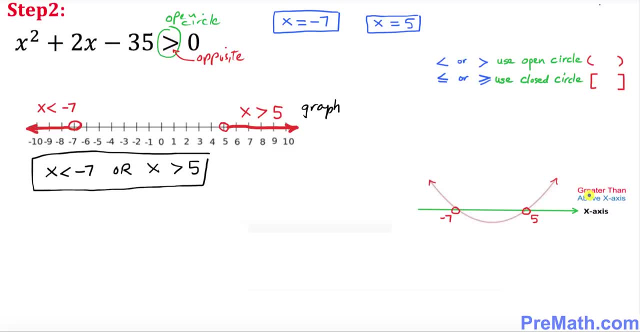 that we have inequality greater than Always. whenever we have a greater than means, our graph is always going to be above axis, If you are looking at above axis means. so this is the part you are looking at. it over here And on this side keeps going on and on, and on. And now, if you want, 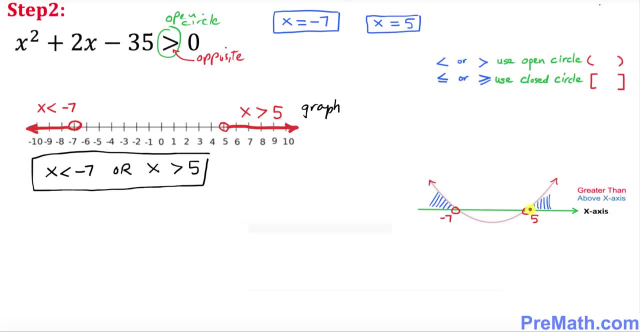 to look at it on this number line only. that's going to be only this part, isn't it? This part And this part as well. So no wonder. I put it down, this on the real number line, this graph, And also, if you want to put your solution in terms of set notation, it's not really hard.